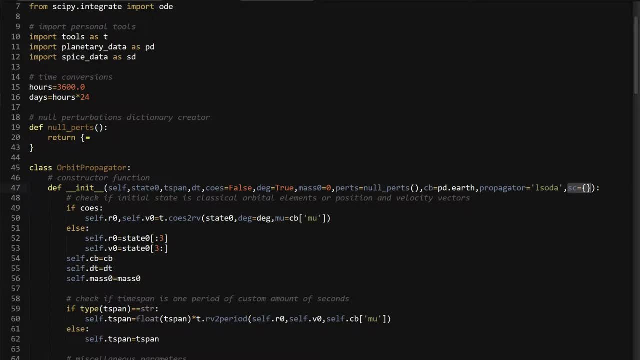 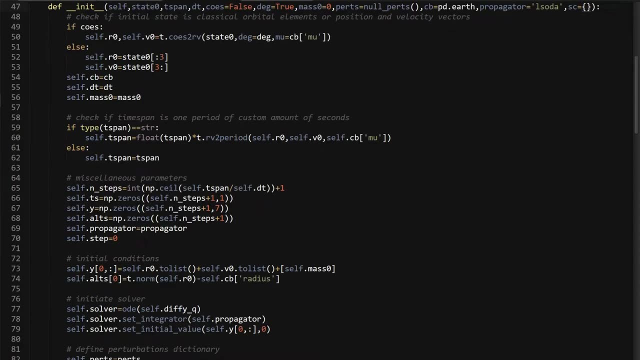 That's just going to be a dictionary that you're going to pass in that has all the stop conditions that you want, And then as default, it's just empty. So that's that. And then another thing that I changed because of the selfstep variable. 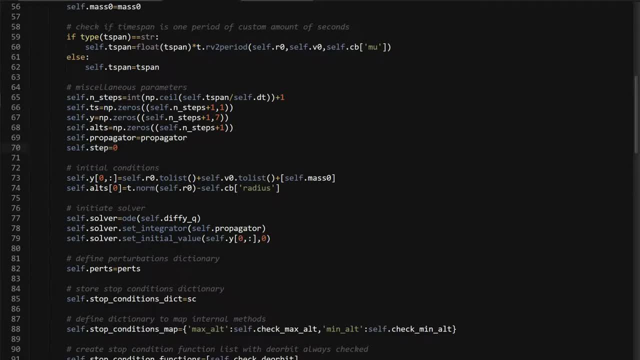 First of all, I changed this to zero, and I'll show you why. But then I also initialized the altitude array here instead of calculating it after all the propagation is done. I'll show you why that is as well. And then I added a plus one to all of these. 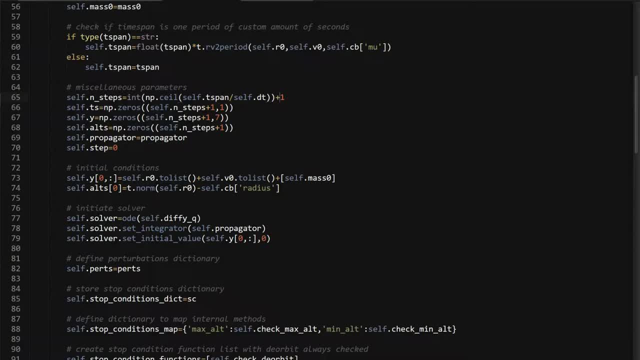 So you want to add a plus one to all of these- This plus one was already here, but to these specifically, And I'll explain why I did that. And then, since you're defining the alt here as zeros, you want to go ahead and define the initial condition as well. 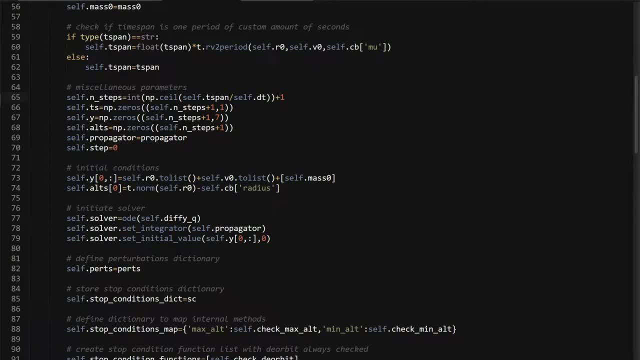 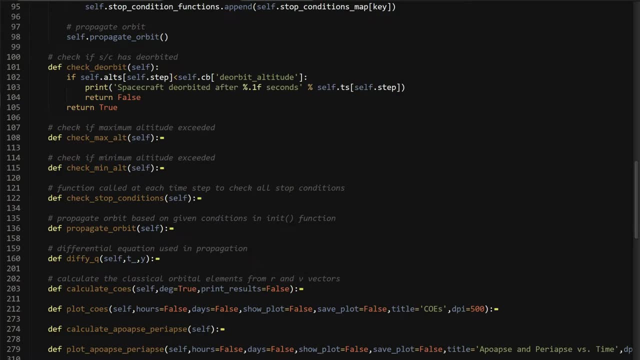 Which is just the same as before, just the norm of your radius vector, radial vector minus whatever central body radius you're at. And I'm going to show before how I do it in the init function, how it's used in the propagate orbit function. 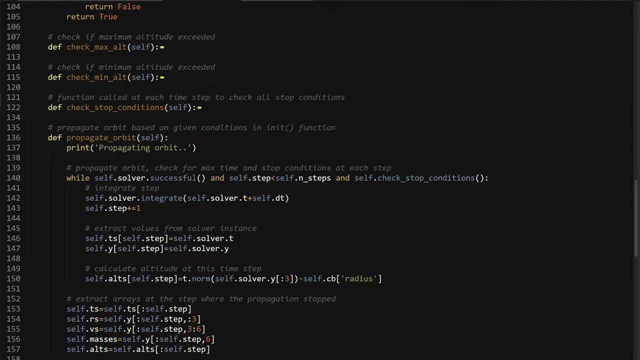 I'm going to hide this. So in this one, where previously in this while loop is going to be: if a solver is successful and you haven't reached it, I'm out of steps, keep going with integration. But I also added successful steps and then if all the stop conditions say to keep going is basically what that's saying. 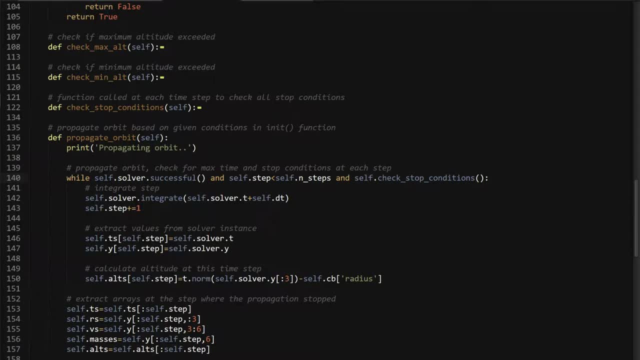 So if everything is true, then you go forth. If any of them are false, because it's and, and If any of them are false, everything will be false and you get out of the loop. Extract the values. Oh, and I moved step plus equals one to here because we need the altitude at the kind of current step. 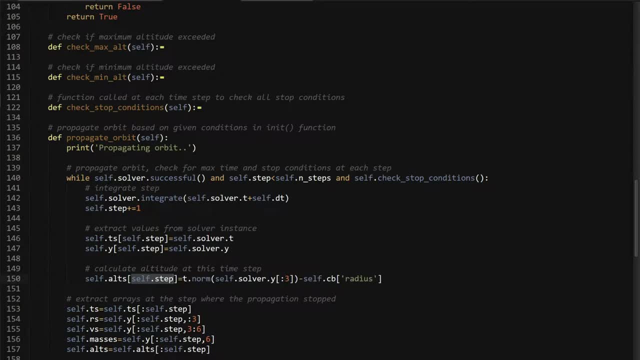 That's going on, so I couldn't have the step be after. that is something I changed for this and I can. I'll show you the old version of the way I had it, where everything, more so, stayed more the same. You just have this other class, but I want to do this one for now because I like. I like this way better. 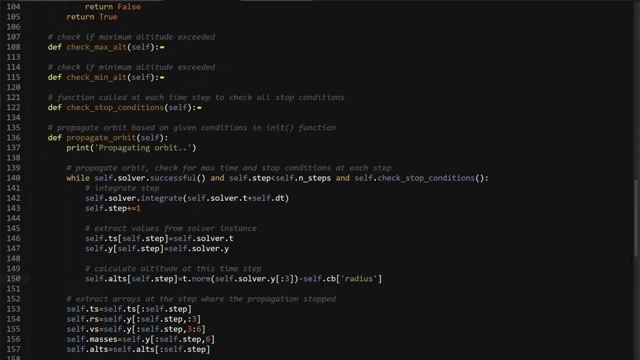 So then you calculate the altitude at your given step and then you norm, And the reason you have to do this kind of first is because you're calling in the previous step or in the step that just happened. Um, I guess right after you propagate, um, check, the stop condition was met. so it's kind of just like that one offset in order to go into the next step. that may have been a little bit fuzzy. 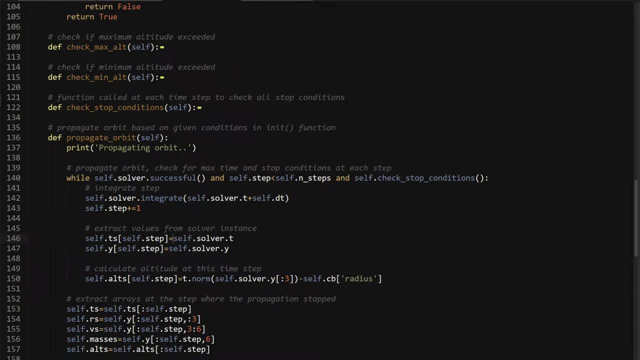 Uh, let me know if it was. but um, I can explain it more if you need to. but um, that's kind of what's going on here. and then use the same as always: Just calculate the norm of your real vector minus the radius and add that into the altitude um array and then at the end just make sure you also cut it off at whatever step. 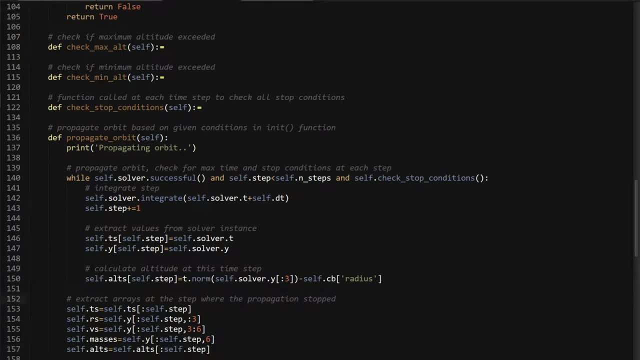 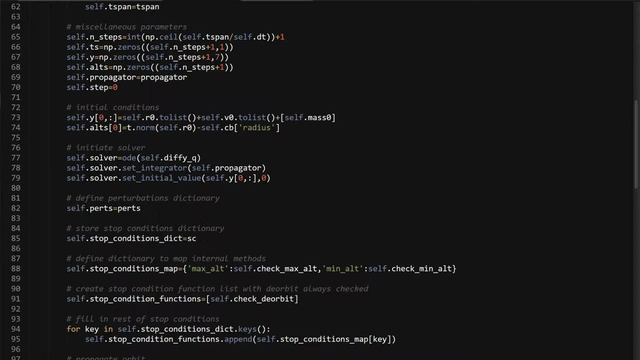 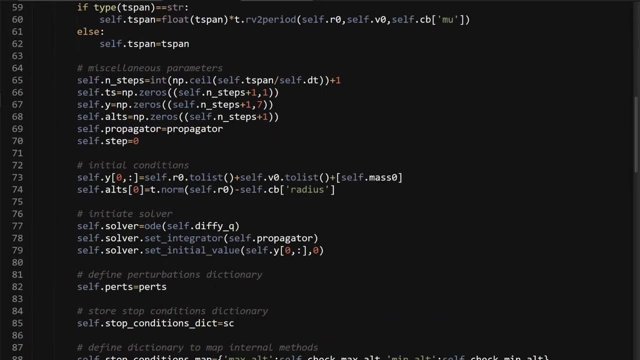 It was. It was cut off, um, just like all the other ones. Um, yeah, so that's it for the propagate orbit. So, as far as what I did in the init function, which is the most important, um, so, this SC dictionary that you pass in, uh, first thing I do is just store it, um, just store it right here as an internal variable. 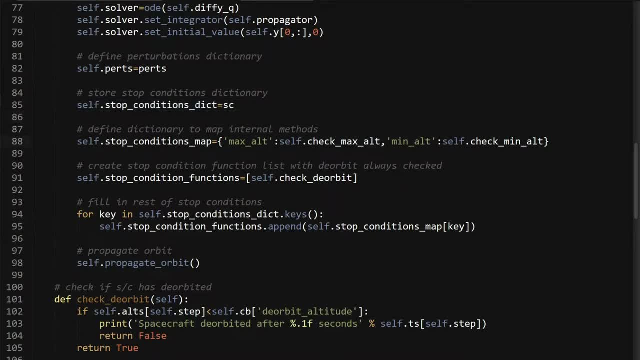 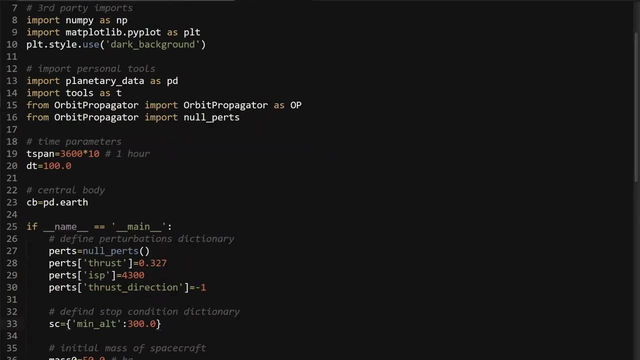 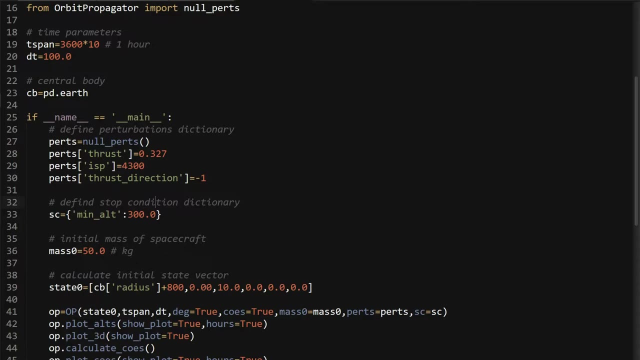 So you always have it, Um, and then this map, kind of this map dictionary, is basically: so, this dictionary, what you're going to pass in, Yeah, Just say, um, you have a minimum altitude. So if you hit 300 kilometers you're going to stop and you're passing in mid alt and then 300. 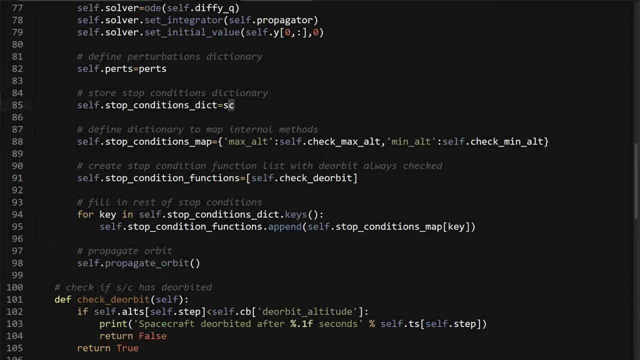 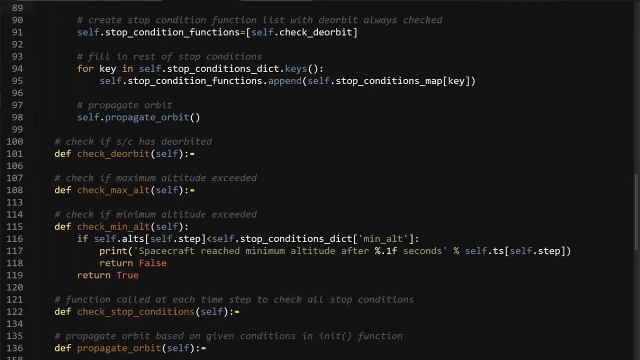 So what's this going to do? Is it saying: um, it kind of maps a string to a function. So for this middle say, you want to do minimum altitude, checkman, alt. So this function, checkman, all it does is if your altitude at your current step is less than what you pass at the minimum altitude. 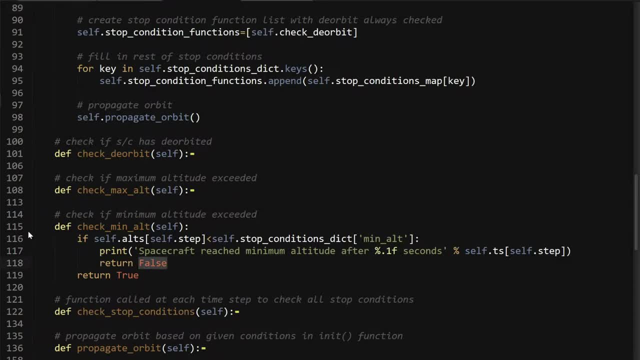 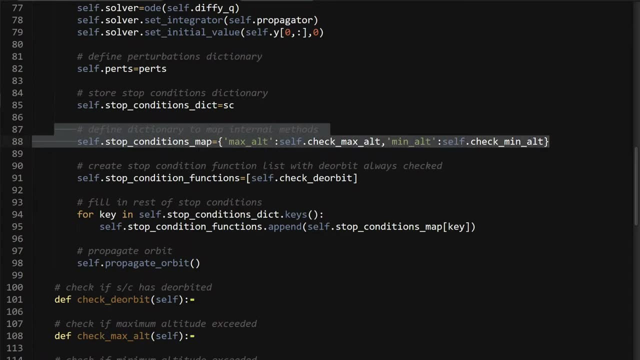 Yeah, Reach minimum altitude- return false. So that stops propagation. So that's what all it's doing is just mapping a string to a function. That's all that this is doing, And I'll show you how you use it in just this other line. 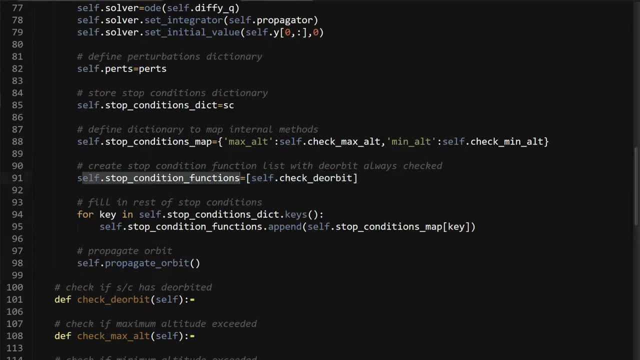 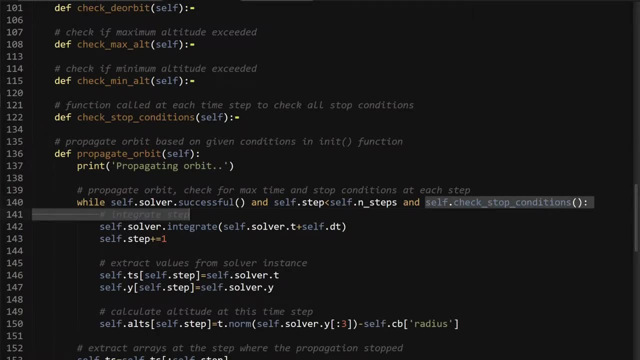 Um so, and then this stop condition functions. is that every step, as it was done in propagate orbit, at every step, you're going to check if the stop conditions are met and if you're okay to proceed or not, and how you're going to do that, is you're going to iterate? 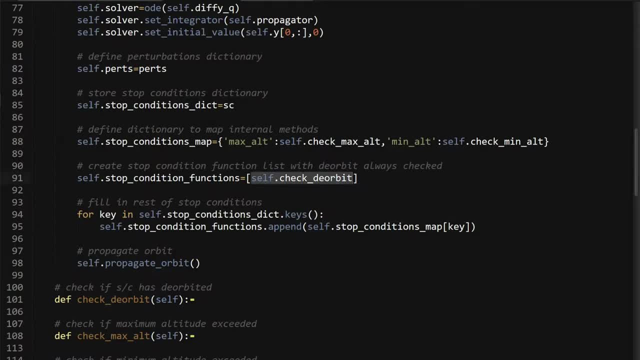 Through a list of functions and you can do this in Python, I think it's. I think you can do it other languages, but it's kind of a Python thing to do, to make a list of functions and then call a list of functions. 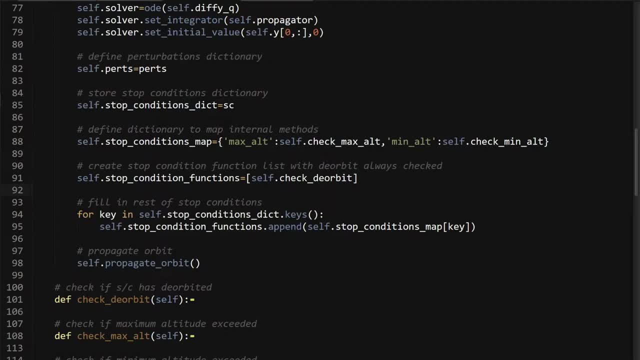 Um, Python just gives you a Liberty of doing that, and it might be possible in other languages, I'm not sure, but you can definitely do it here and I take advantage of it. Um, so you're going to initialize this list by always checking the do orbit, because if you do orbit, you do orbit like. you don't want to have to pass in the value every time, because what earth if you're at a hundred kilometers? that's considered. 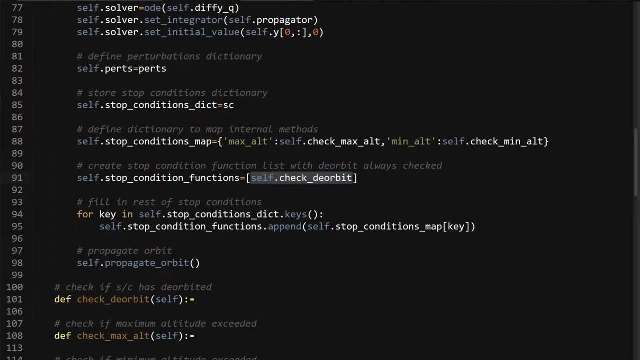 Do you orbit it, So just call it good there, Um, and you can change this value on whatever you want. but so you're always going to check if you do orbit but say, if you're at an asteroid, you're only do you orbit it if you're at the surface. 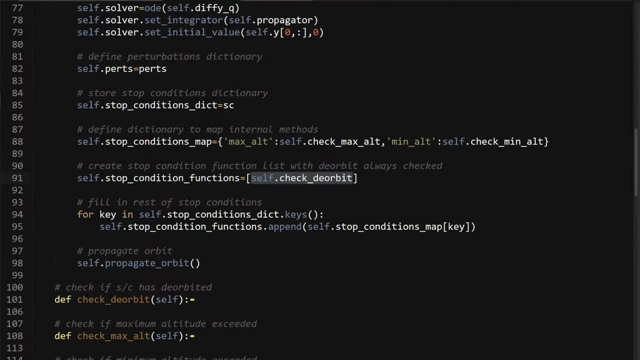 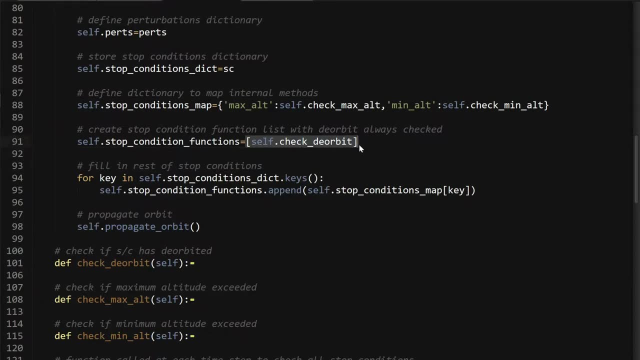 So you can add that parameter as well, And I'll show you how I did it in planetary data file. Okay, So once you initialize this list that just has this value, where you're always going to check if you do orbit, Um, so for key and self to stop conditions. Dick duck, he's Dick. 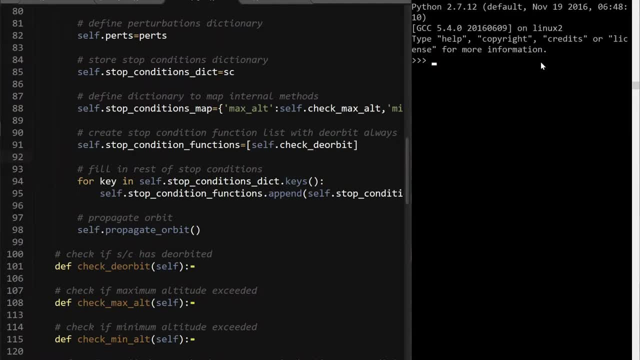 That's in dictionary. So, um, what you can do is see you have a. this arbitrary dictionary just says like min alt, um 100, and then you say max alt, uh, 1000.. So what this keys? so a doc keys just returns you a list of strings of the key. 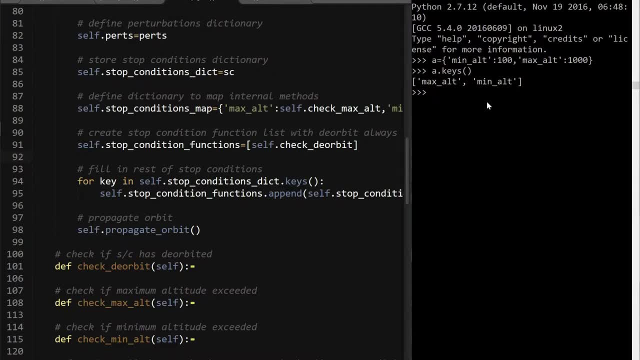 So this is key and value, key value pairs. So I think, if you do, is it values? Yeah, It returns you a list of Whatever values you had. um, oh, you just, I guess, make sure it doesn't matter what order you pass them in. 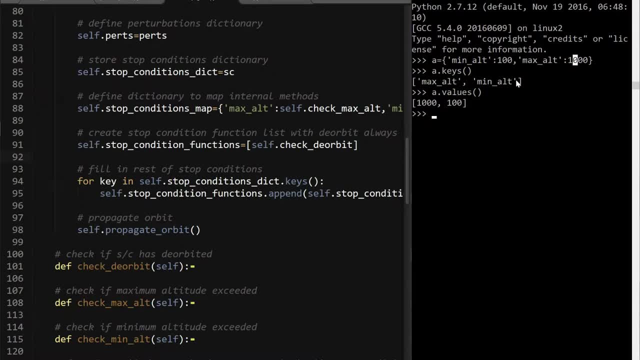 I think it does it alphabetically um or whatever algorithm it does, if it has, because you can also do um. say you have one equals Yes, And then if you have a you can have, so you can have a lot of different data types. but that's also a very Python thing. 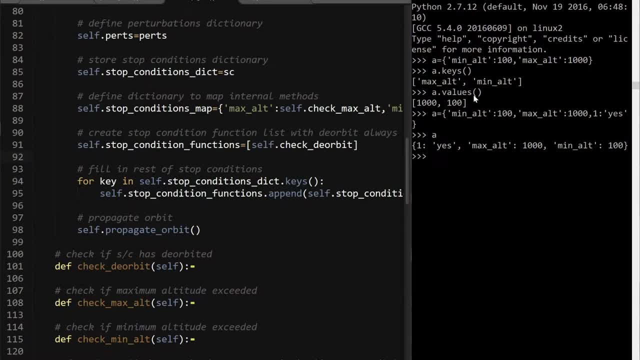 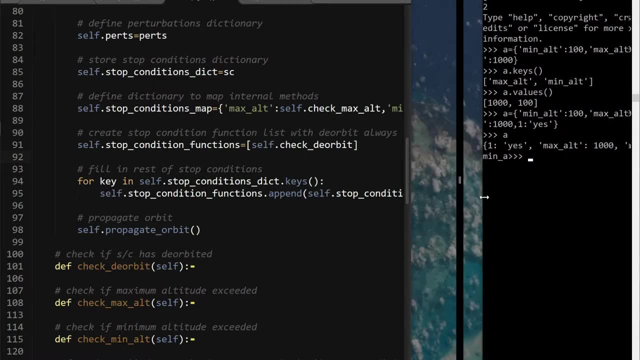 You just mix up data types however you want, Um, but they're not gonna be alphabetical, So but they will be in the same. if you do keys and values, it will be the same anyways. Um, what I want to get from that is that when I say for key and self dot, stop conditions, dictionary dot keys, um, each key. 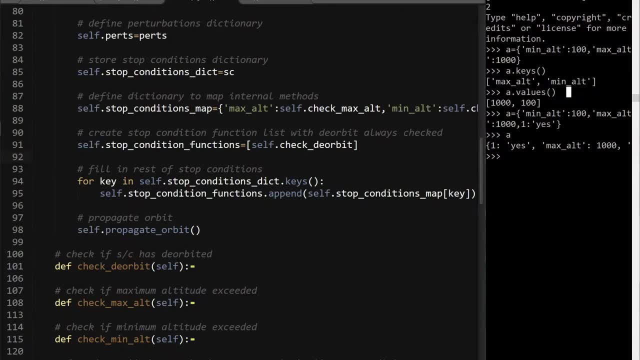 So you're going to get max, alt, min, all and then whatever else you want in there. I only implemented these for now, but you can implement literally anything you want. Um, so you're going to append to this, that's this list. uh, whatever keys you pass in, you're going to append, um, whatever function that maps to. 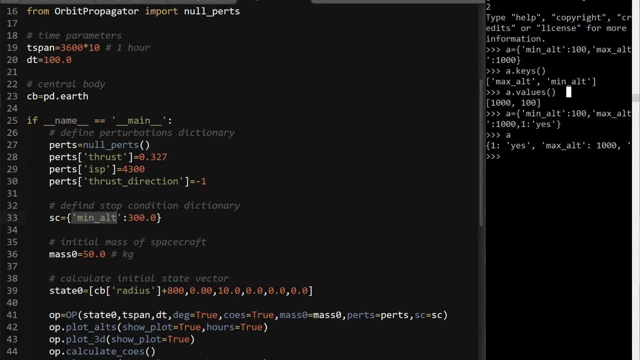 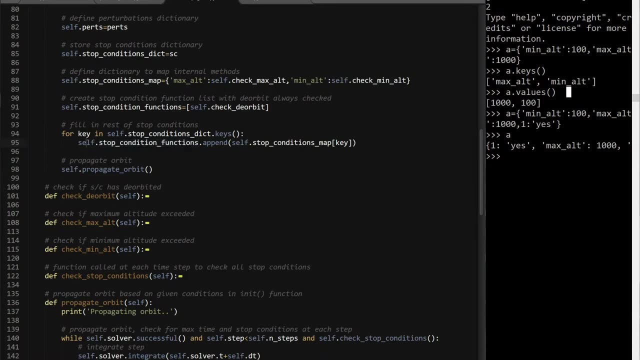 So in this, in this first example, you have Min alt and you want a 300. So what that will do is you have um. since one of the keys in those dictionaries is min alt, it's going to get min alt. 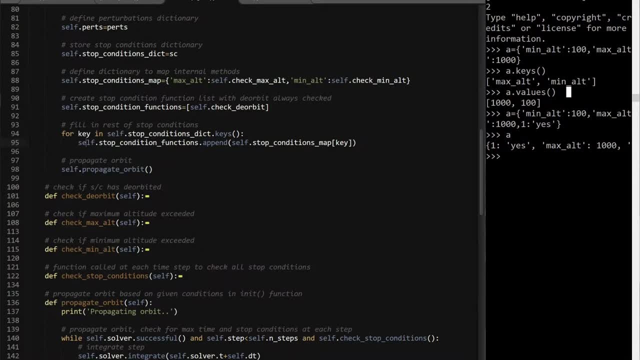 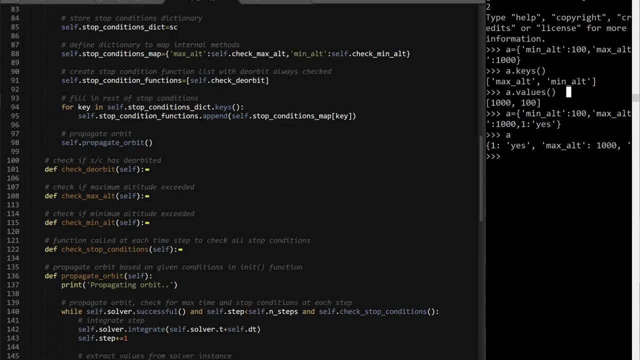 And then from this, it's going to append to this list this function. So every time that this is called here, it's going to check if the minimum altitude has been reached. Um, there's kind of like dictionary stuff going on there, but um, it's kind of a more efficient way, in my opinion, than what I did. 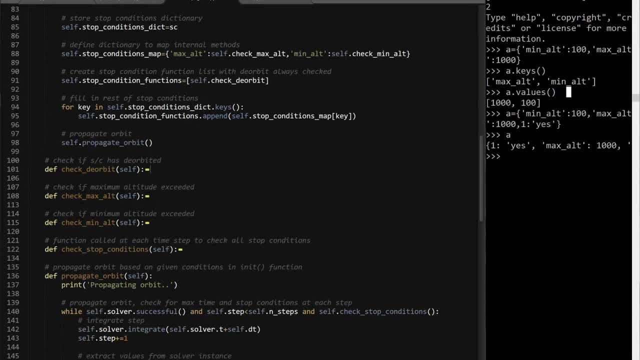 Before which I'll show you. um, but that's just what's happening here. So you're going to fill in the rest of the stop conditions, You're going to add the rest of the methods inside the class of the stop conditions, inside of this list. 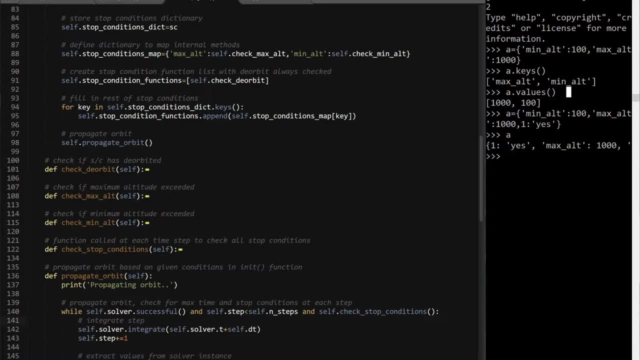 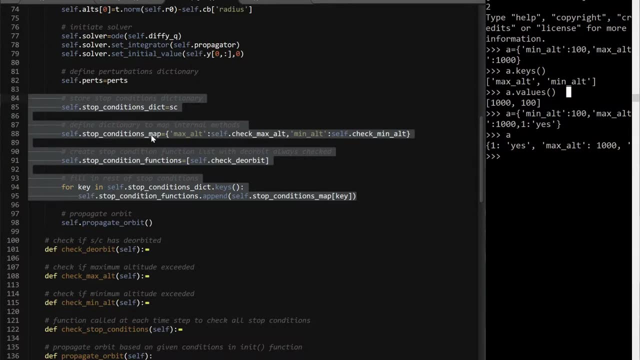 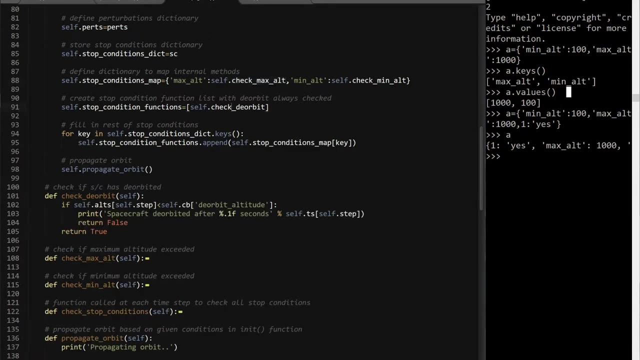 So each time step, it will check if those have been met or not. Um, so that's what's happening there, and just these uh kind of four commands are what you're going to add in order to add stop condition. And then, as far as these functions, um, first of all, check the orbit is basically if self dot alt. 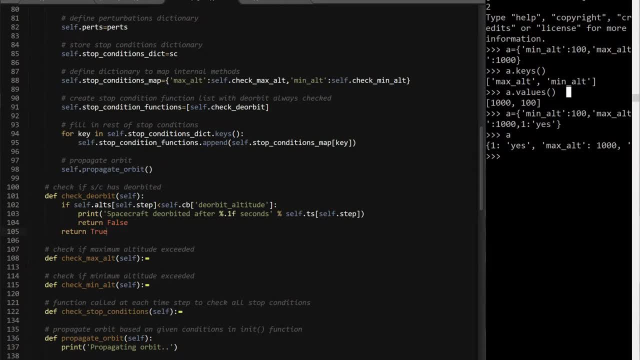 So If, If the altitude of your current time step is less than deorbit altitude, it's deorbited, and I print out a statement and then return false, And if this is not true, you can return true. One thing worth mentioning is, um, I could also say else, return true, and there'd be literally exactly the same, but I just decided not to use else because I don't know less writing, I guess, um, because this is true. 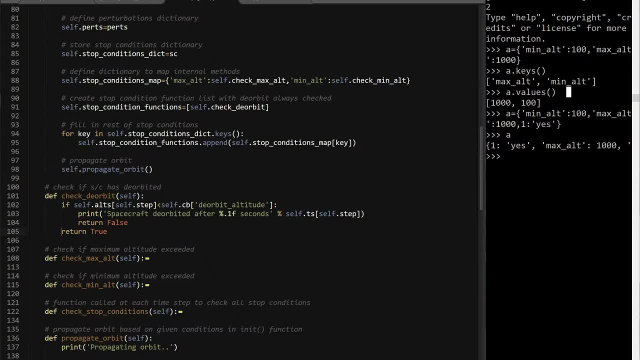 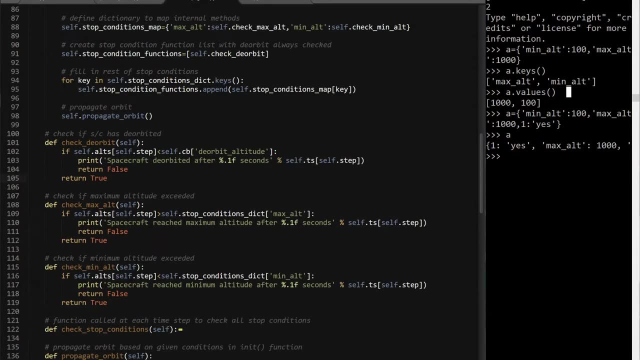 It's going to return. It's never going to call this line. So if you return, you get out of function. So it's never going to call that And then. so right now I have implemented max Alt and min alt. uh, max altitude, minimum altitude- pretty self-explanatory. 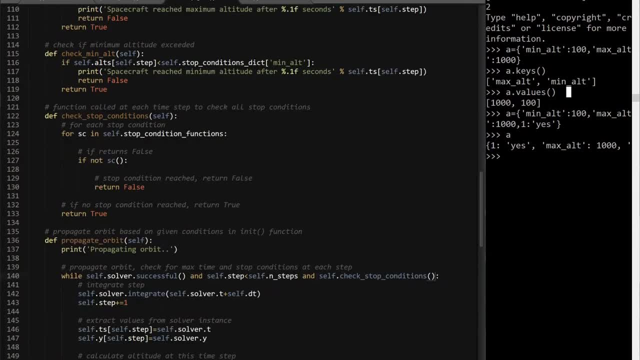 And then this: uh, the function you call here is self dot check stop conditions. So that's this function here, Um, and what you do, So for each stop condition, so for SC stop condition and self dot stop condition, functions which you define here. 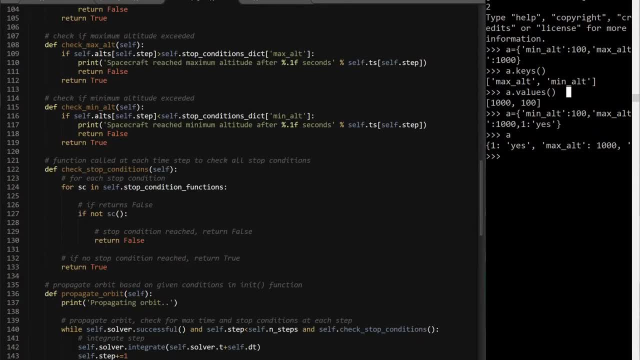 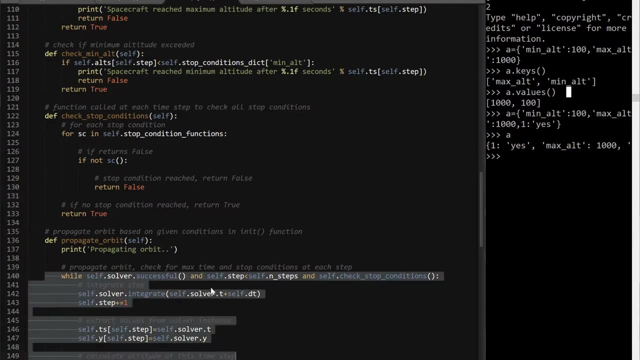 So for each function in this list, call it. So this will return either true or false. So if it's not, if it's not false, which means if it's true, then some stop condition has been reached. return false. And when you return false, you get out of this loop. 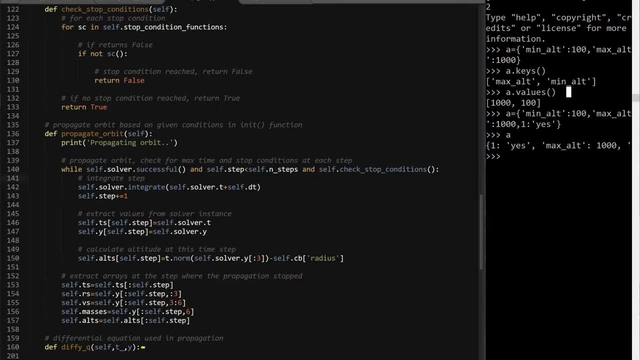 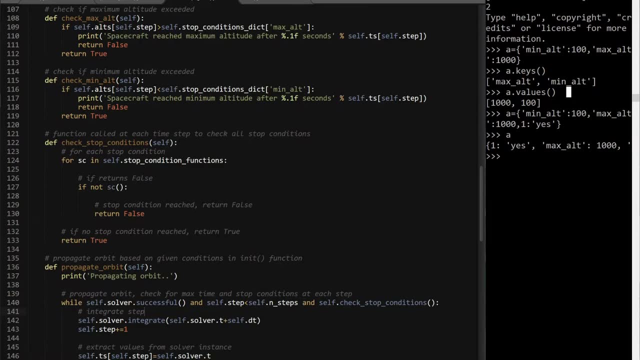 So you stop propagating and then you cut off all your arrays at whatever time step you stop propagating. So what's going on? Um, it may get a little, I guess, confusing with all the Booleans going around here. Um, so just let me know if it is. uh, I can, you know, give a little bit more explanation as to what's going on? 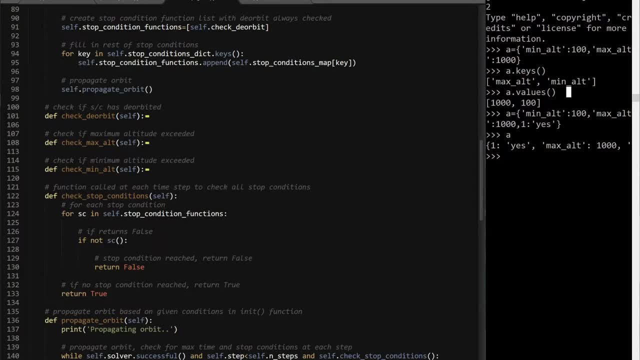 Kind of the mapping is what's going on, But there's a lot of Booleans, But, um, I think I mean, at least in my mind, I don't know. if you think through it, they kind of all make sense, but please let me know if it doesn't. 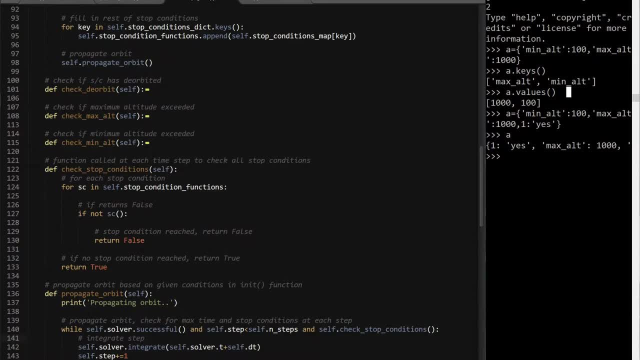 Um, so, for each one of the stop conditions, if one of them returns false, return false, the stop condition has been reached. So if you never returned false, that means no stop condition was reached and returned true. So then this will return true. 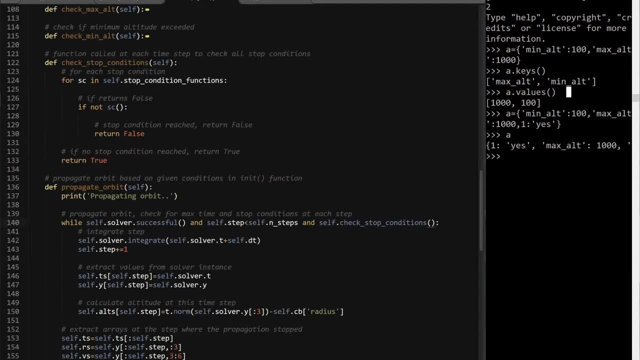 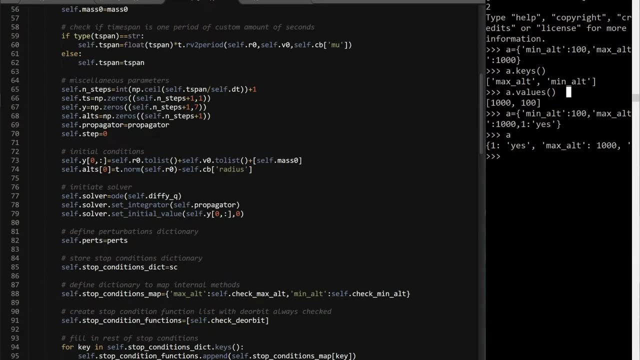 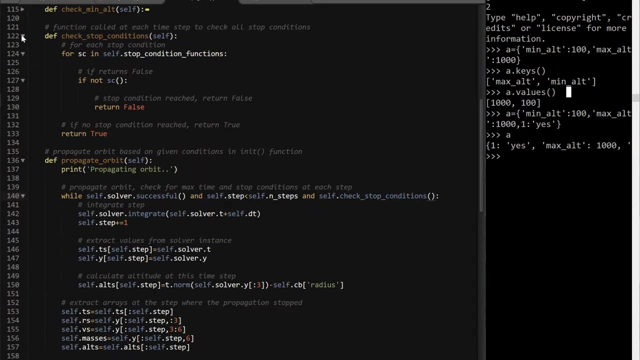 And then you keep going with the propagation as before, as if nothing happened. you're just checking if some stop condition has been reached. Yeah, that's kind of a lot to explain there. But um, yeah, again, let me know if I need any more explanation on that, because I actually just wrote this today when I was making this video, kind of just thinking about how can I do this better. 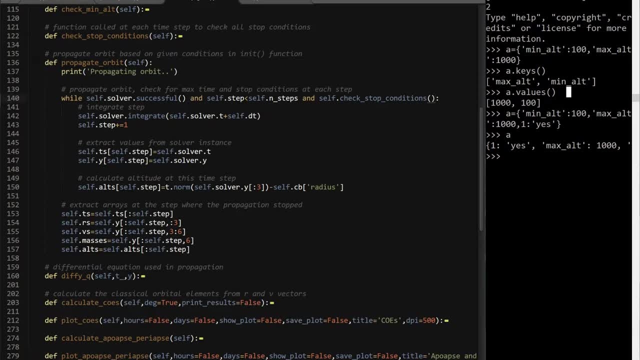 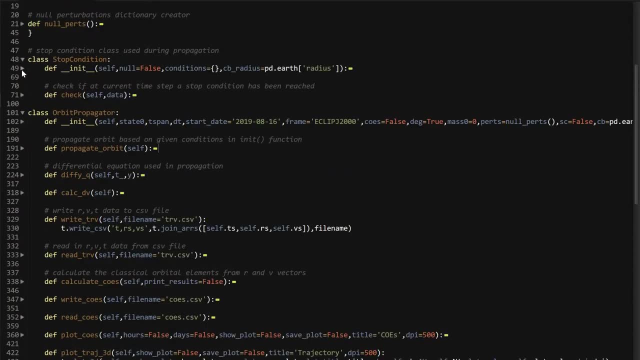 Um. so to cover what I did before, which also worked when I had the stop condition as a separate class Um, here's a stop condition, class Um, where you initially pass in a null equals false. So if there was going to be no other stop condition, 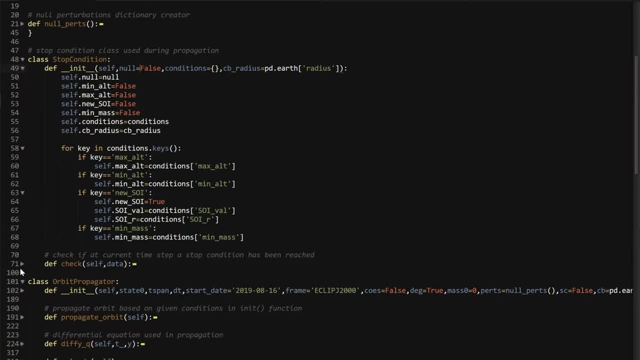 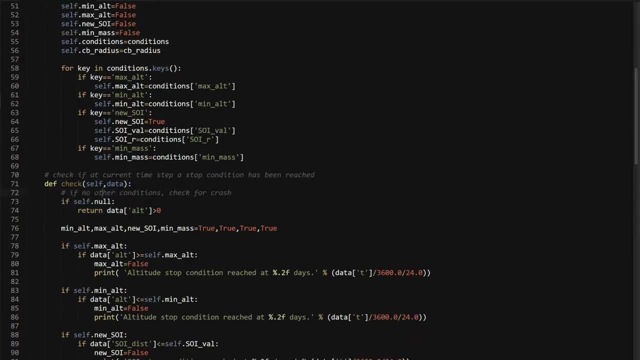 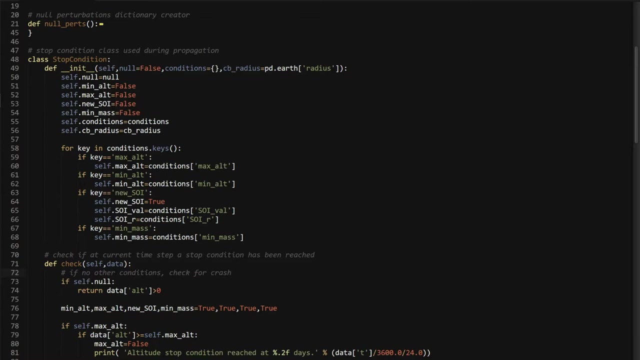 There's going to be no other stop conditions other than checking if you've um crashed. Basically I used to have it if you've crashed, If no other conditions check for crash Um, just do that Um and then for each uh kind of um stop condition that you would have, you would pass in true or false. 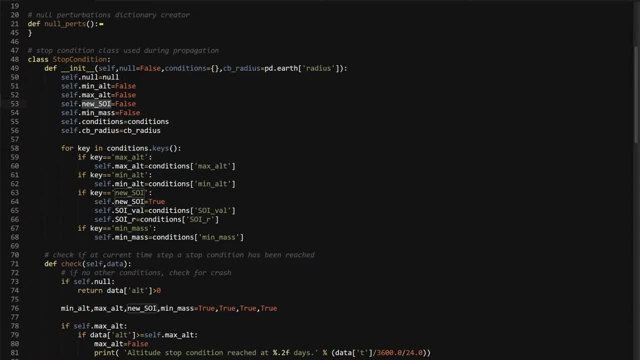 So minimum altitude, maximum altitude, SOI sphere of influence. So I use that one, for if you're leaving Earth and going to the moon, at some point you're going to enter the moon's uh sphere of influence, So just trigger that when that happens. 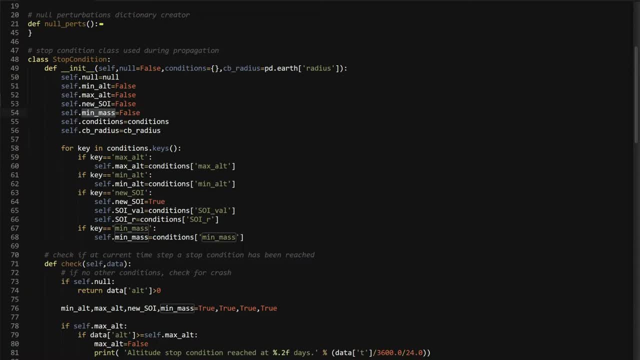 And then min-mass. So if you only want to use a certain amount of mass, um when you're thrusting, And then conditions equals conditions. So I still passed in the um dictionary And then so I would pass in whatever central body radius was going on. 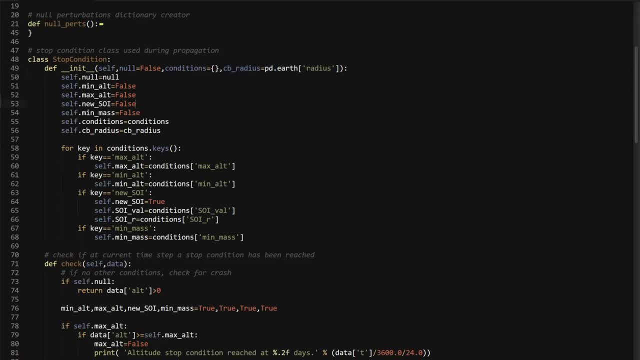 Um, as a default, it was Earth. The problem that I had with this was: well, I actually didn't have any problems, It worked just fine. I just I really wasn't a fan of how many if statements I had. 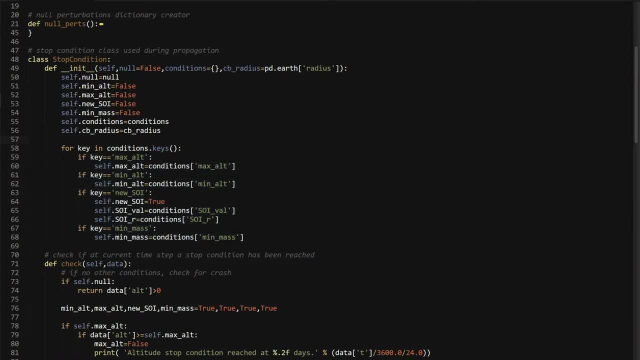 I'm really not into. I try to kind of do as little as I can Do, as little if statements as possible, But obviously I was getting a lot here. If you're passing in max-out, set selfmax-out to be whatever it is. 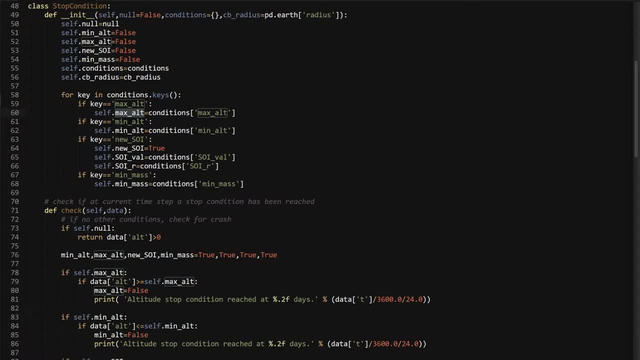 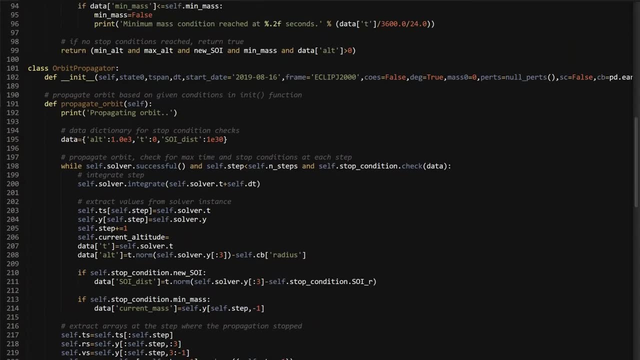 Blah, blah, blah, All of those. And then what I did was, in the check um, I had a method called check, Which was used in propagate orbit Um, where I used this selfstop condition, So I would pass it in. 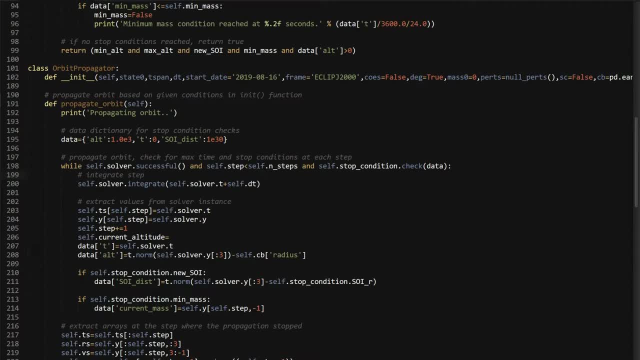 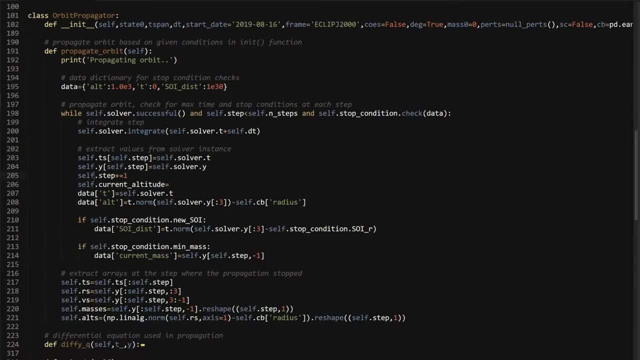 And then it would store the stop condition instance as a variable And check And you'd pass in a data dictionary. So I didn't like this because, um you, you're creating a new um variable, basically, And you're passing into this function every time. 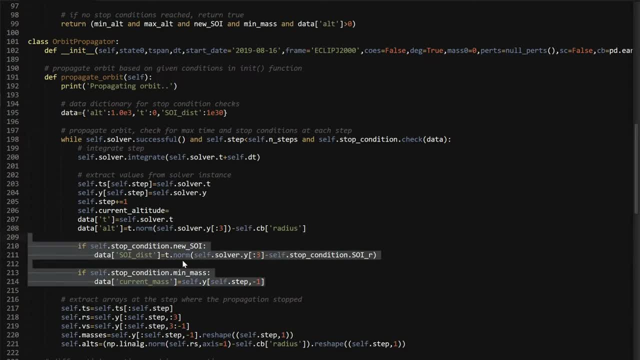 And then here's two more if statements. So if you're checking for a new sphere of influence, add it to the data dictionary And then pass it in. So I just kind of just didn't like that. Um, I had this as well. 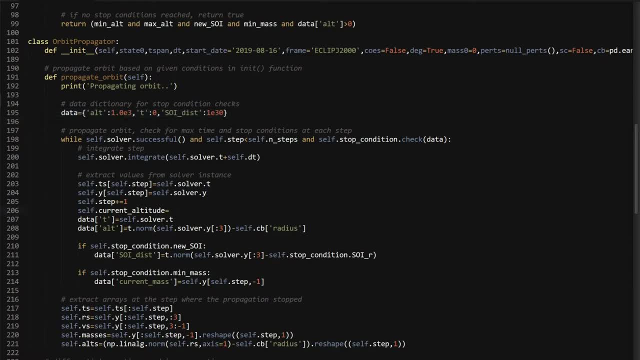 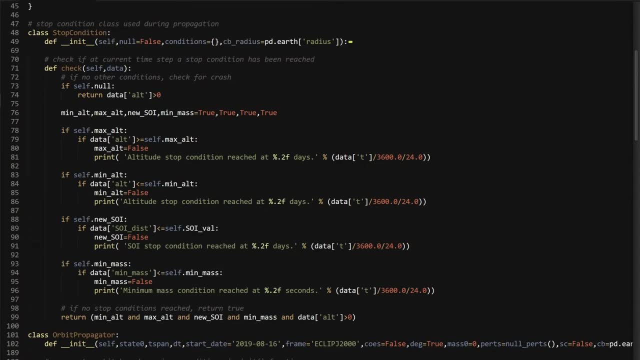 You had to initialize that. Um yeah. So I just kind of thought there has to be a better way, At least in my mind, Um a way that makes more sense, And then when you check, you have to initialize all these to true. 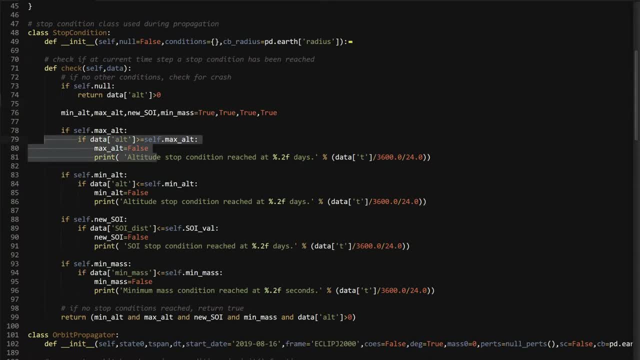 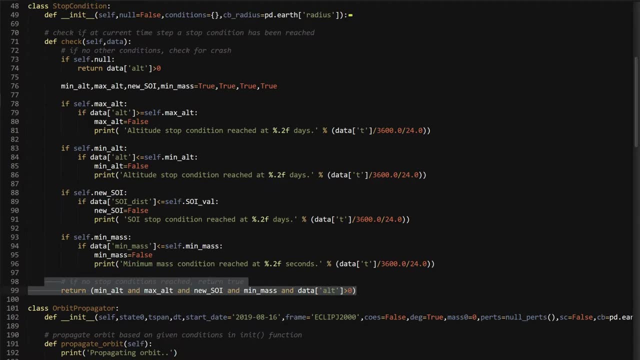 And then, if something is false, flag it as false And then, at the end, return all these ands. So if any of these are false, then you return false, Because these are all ands on top of each other. Um, yeah, 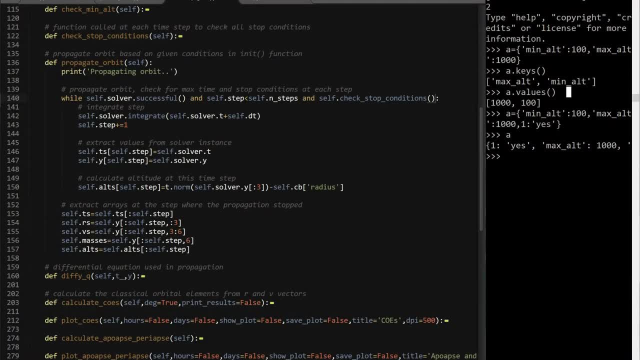 It's just the way I had it before. I just didn't like it as much And wanted to redo it, And I feel like this is a more efficient way of doing it, Um, especially because I just really don't like having too much of if statements. 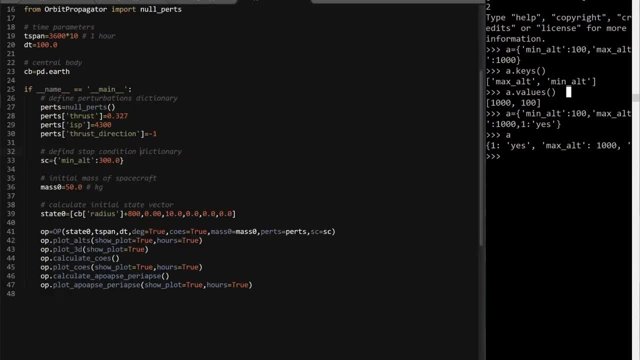 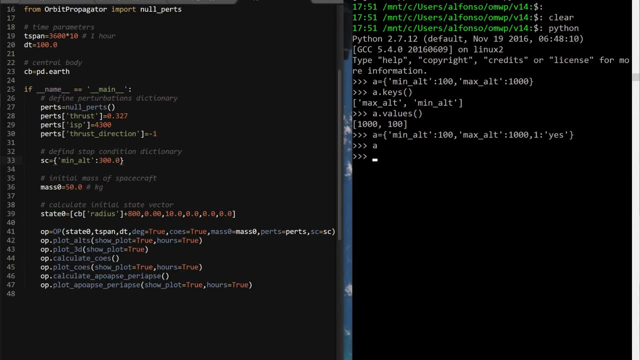 Yep, So I think I can just move on to this now, And I already ran this, So I know it's going to work. But basically what's happening here is I have this initial orbit that I had with 800 kilometers Um, it's basically circular. 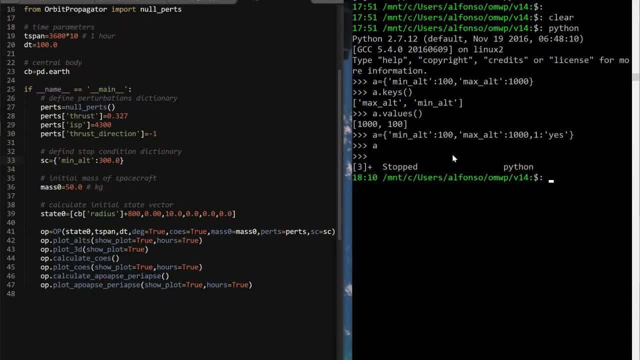 Oh, it is circular. I put 0.0 for the eccentricity And then I'm just going to run it and show you what this looks like, Where I had the minimum altitude be 300 kilometers, And I'm thrusting in the negative direction. 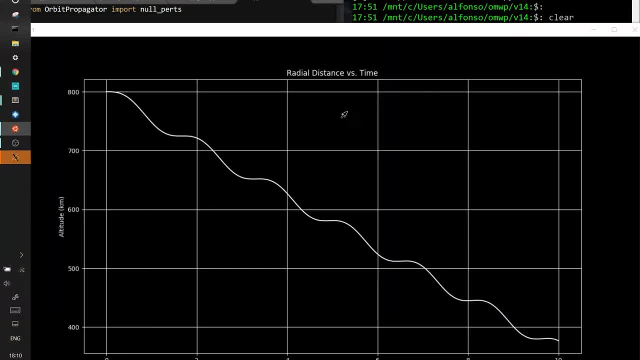 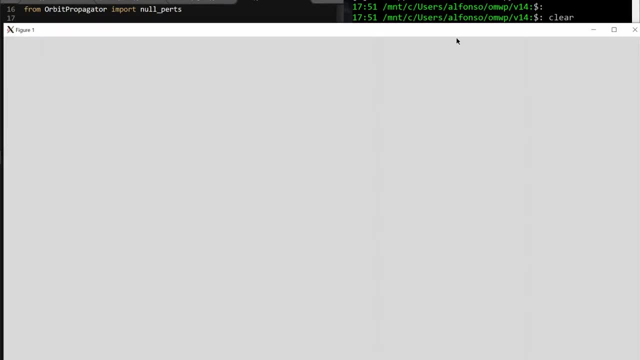 So that means I'm trying to de-orbit. So, as you would expect, you get down here And it just cuts off at 300.. Which might have a better view in another one of these. As you would expect, you're just decreasing in altitude each time you go around. 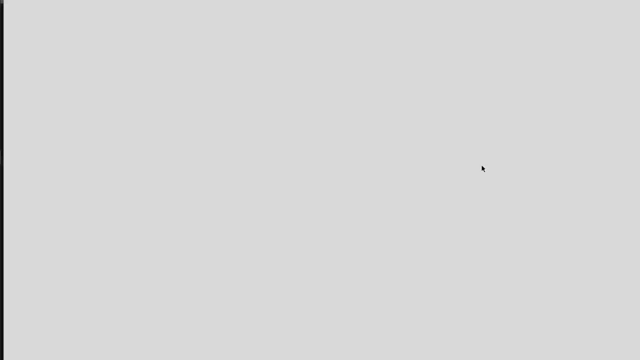 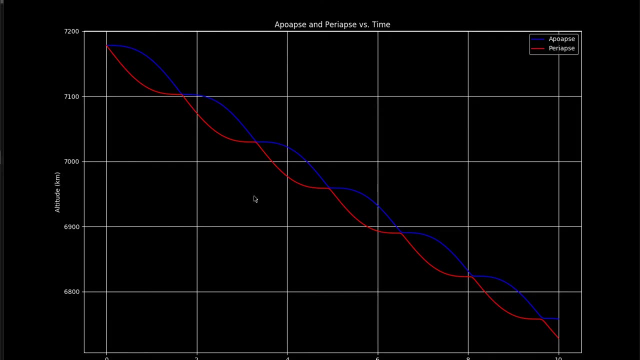 Bottom of the cos. Get to the stop condition. when that happens, This is all pretty much the same thing as before. I just wanted to show you how to implement this. Oh, actually, yeah, One thing that was interesting about this. So apogee, perigee plot. 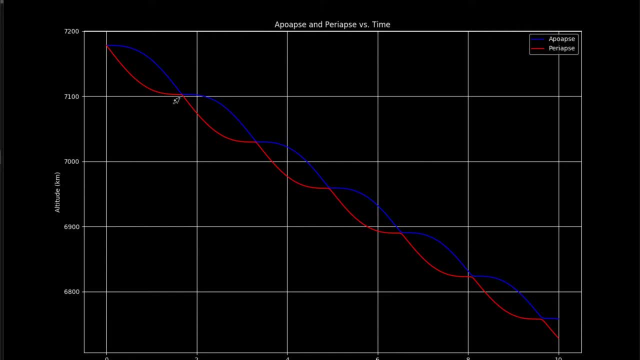 You kind of So. when these meet, this means that the eccentricity is 0. Because your apogee and perigee are equal, You're kind of just bouncing back and forth when you're de-orbiting from a circular orbit. 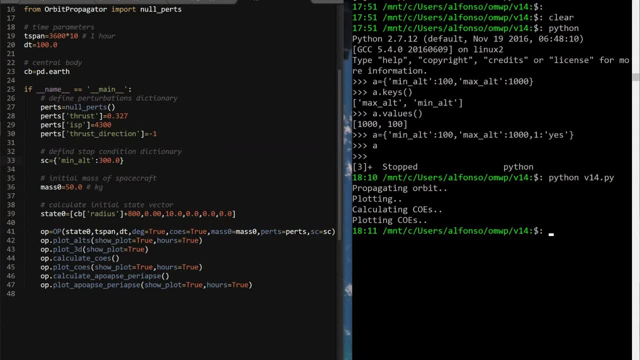 Um, This is going to be different from an elliptical orbit, So I guess we'll just do that. Say this is like a 0.2.. I hope this doesn't crash into the earth. Yep, That's what I thought. 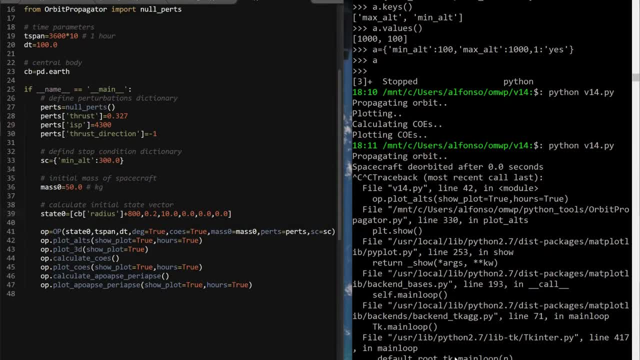 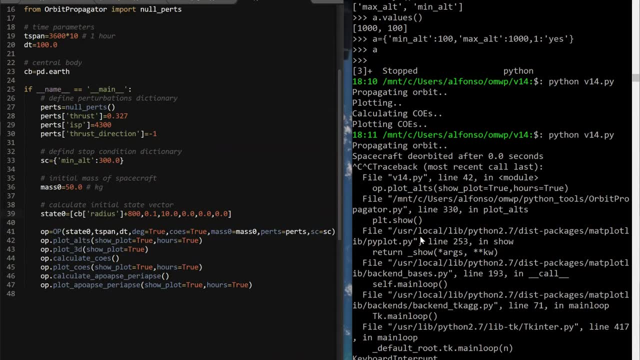 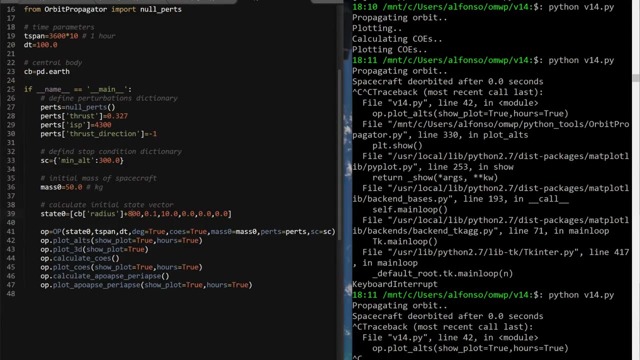 It's just bad initial conditions. Let me do like a 0.1.. And see what that looks like. Okay, These are not the conditions that I want. Let's do like a 1500.. Minimal altitude: of 200.. 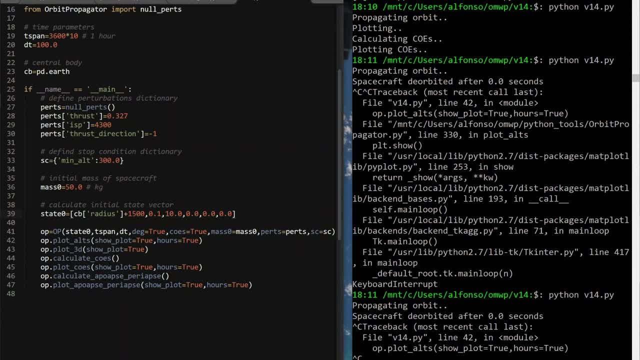 I'm just doing this for Um Kind of just showing sakes, Because the apogee perigee is going to be different. I mean, this is what you'd expect. You're oscillating a lot. Same thing as you'd expect. 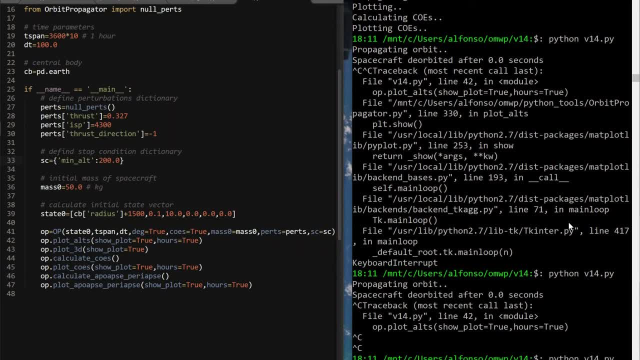 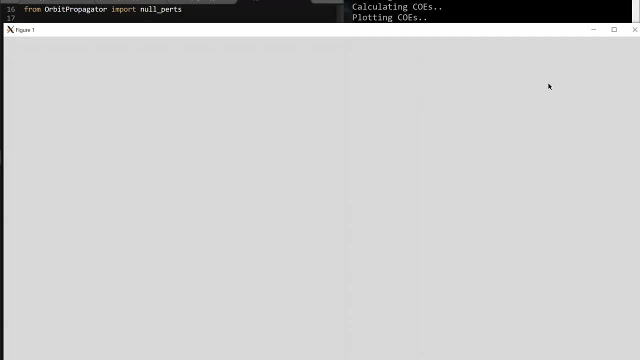 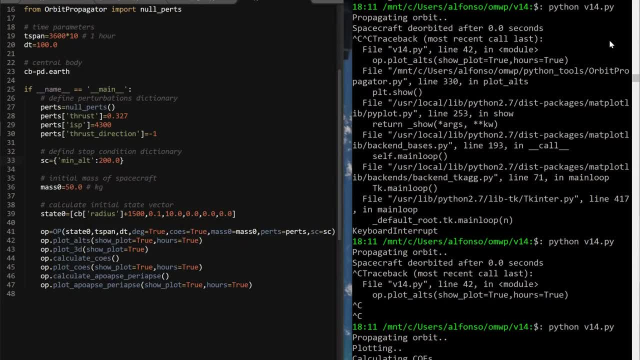 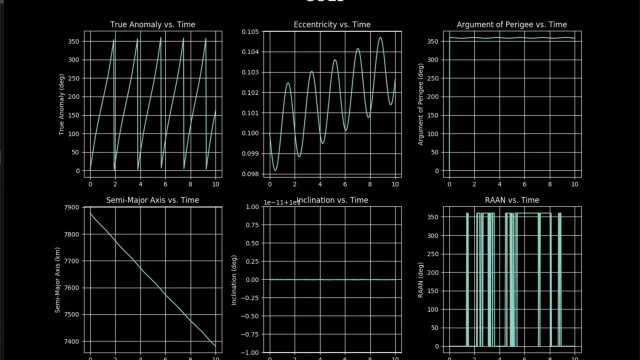 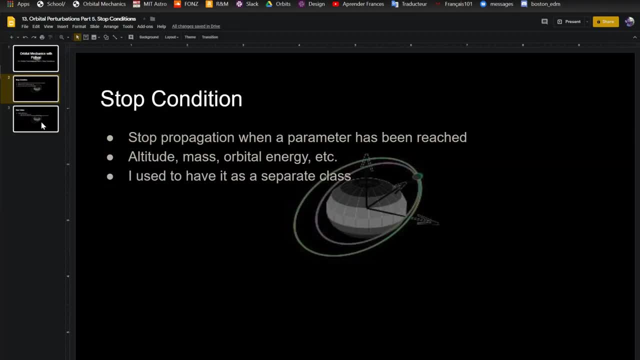 Basically Is what I wanted to show there. So That's pretty much it for this video. I feel like I covered it pretty well. But Again, Just let me know if all the booleans and stuff was a little bit confusing. 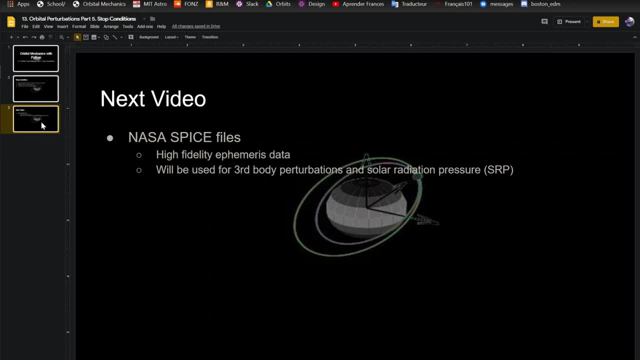 And I can do a better job of explaining. Um, In the next video I'm actually going to start doing the NASA spice files, So I ended up doing three videos, But now I'm actually going to do it, So Yeah, 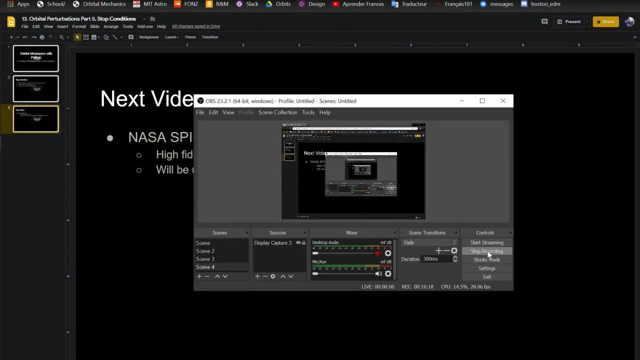 Uh, Thank you for watching. Yeah, Thank you for watching.